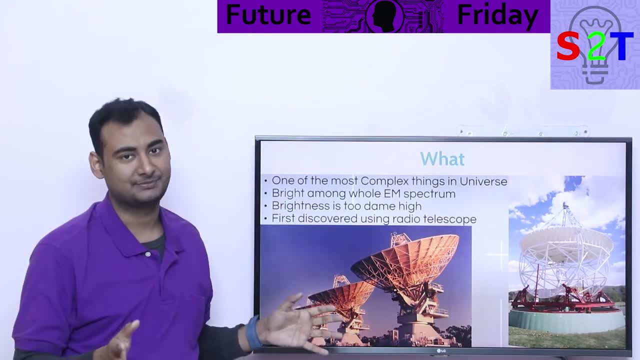 This is the driving force behind it, And there are some things that does not make any sense. This puppy is in that category. does not make any sense. Now it is bright. Now it is a bright object. Now, that's common thing. There are many things that are bright. 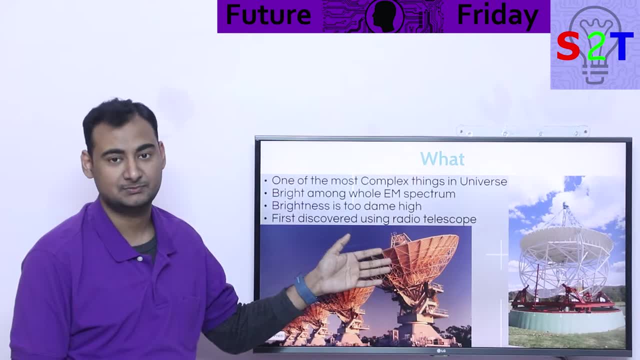 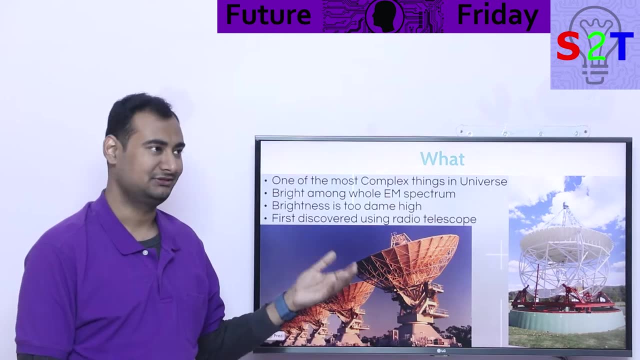 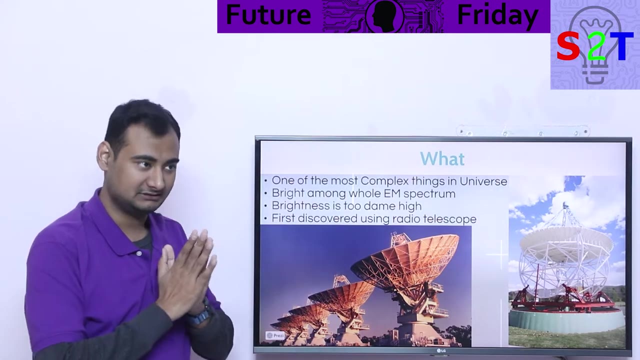 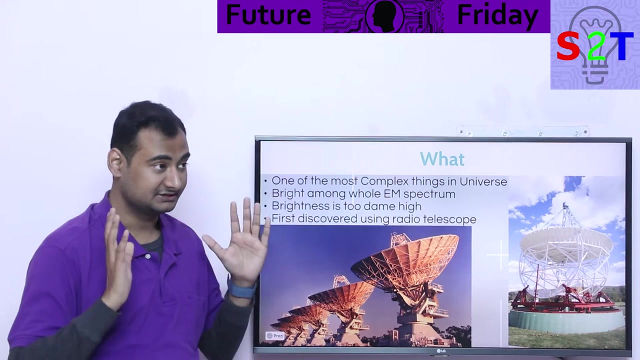 However, this puppy is bright in almost entirety of electromagnetic spectrum. For example, we utilize radio telescope and it was bright. then we utilize optical telescope- we can still see this. then we utilize x ray telescope- we could still see the damn thing. It's like it's bright in whole spectrum. So that means it's ludicrously bright, like for what it is, And radio telescopes were the first clue how powerful these things are. So you have to understand this is a big, powerful thing that is very bright. 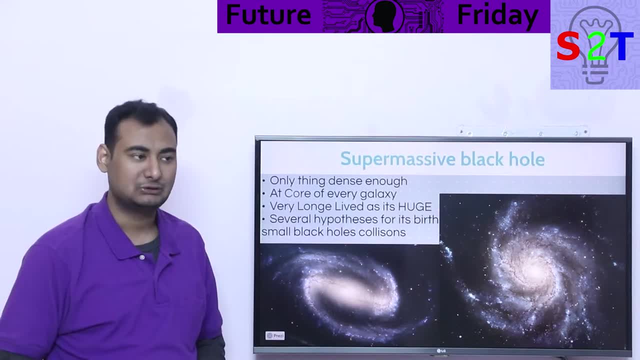 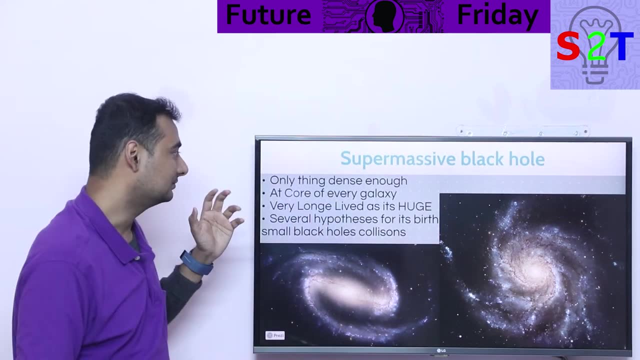 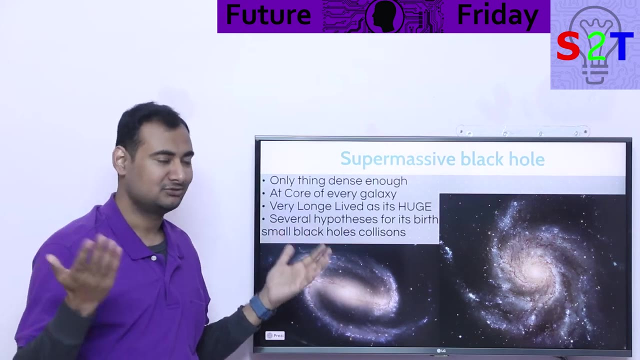 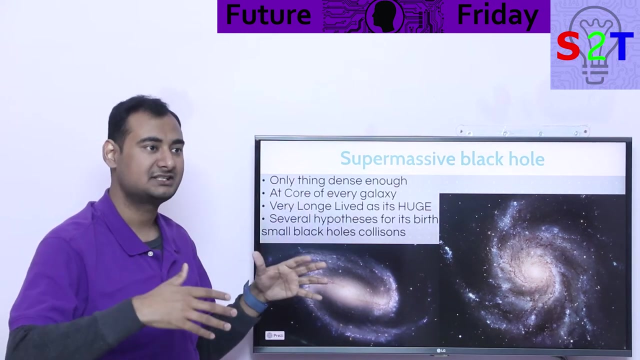 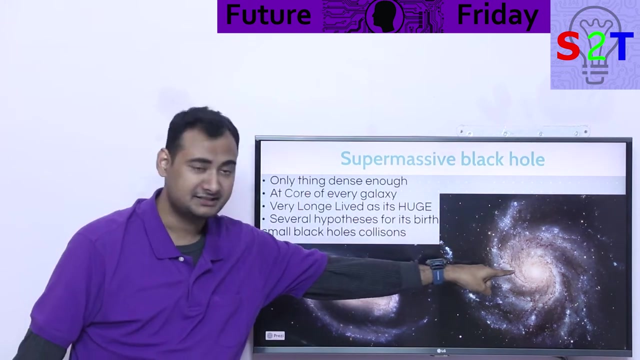 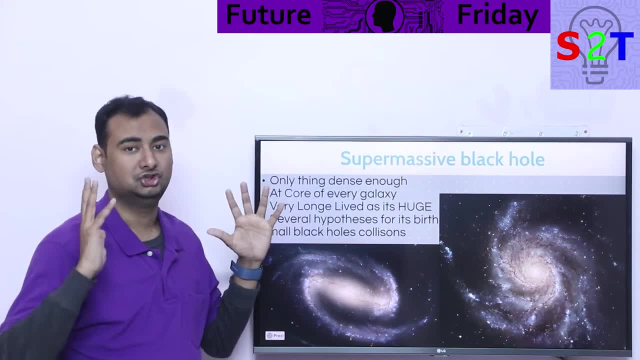 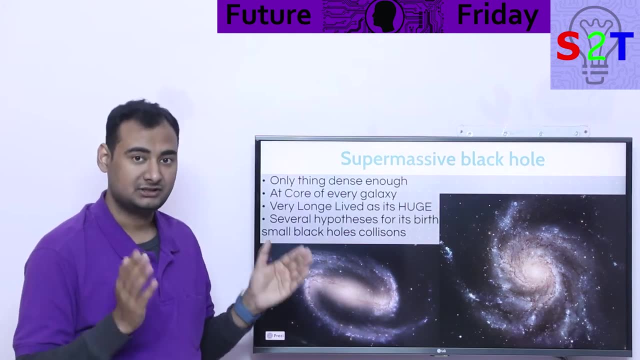 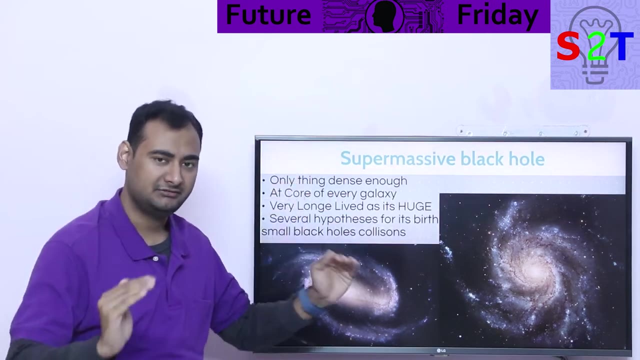 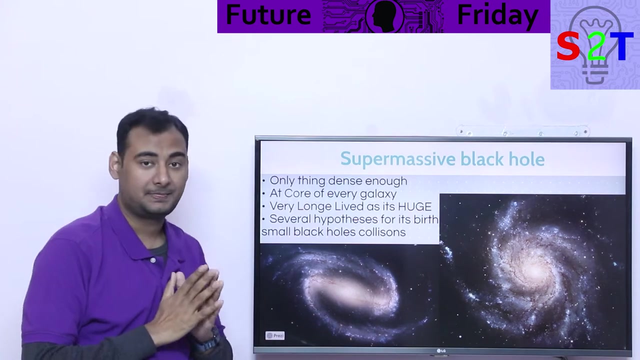 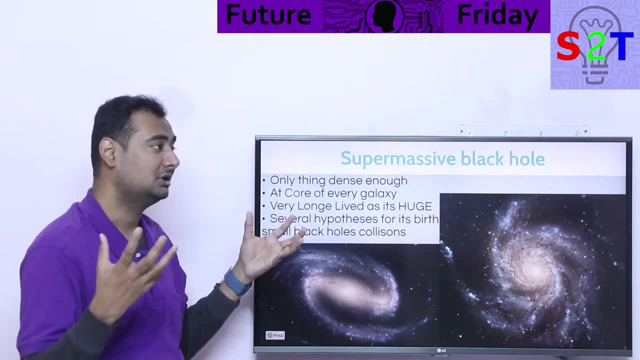 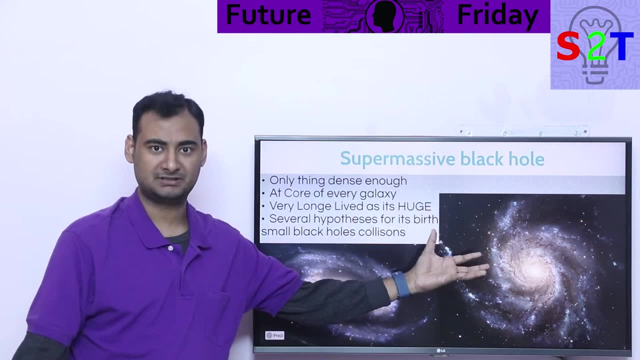 hypothesis. uh, some hypotheses are quite simple, where they are like what? uh, because these black holes while they are in the center, but you will like, how the heck this puppy should be this bright? it's supposed to be the darkest black hole, super massive black hole. the reality is it's uh, basically. 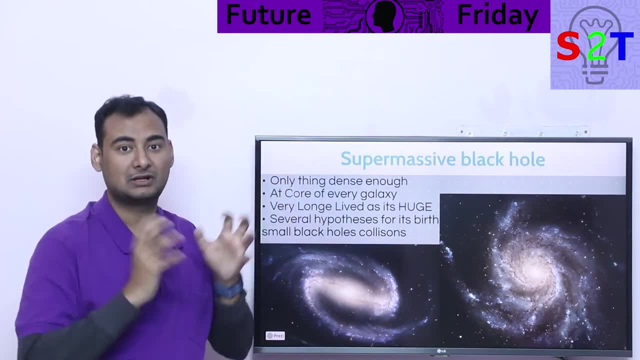 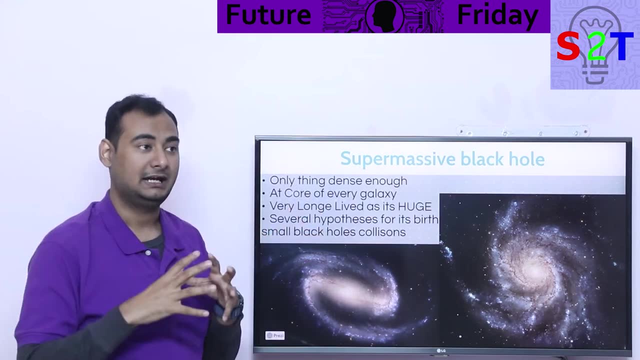 there are multiple stars that are orbiting this puppy. what if all of them collapsed onto it? so, like you know, it will end up feeding it. so if you can feed a black hole and if you are feeding it fast enough, it can start to grow. and the bigger it gets, the basically evaporation rates goes down. 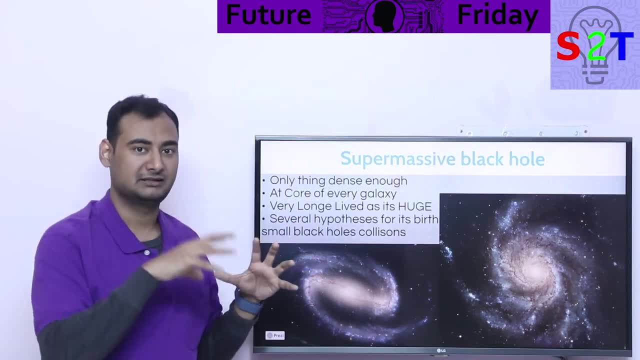 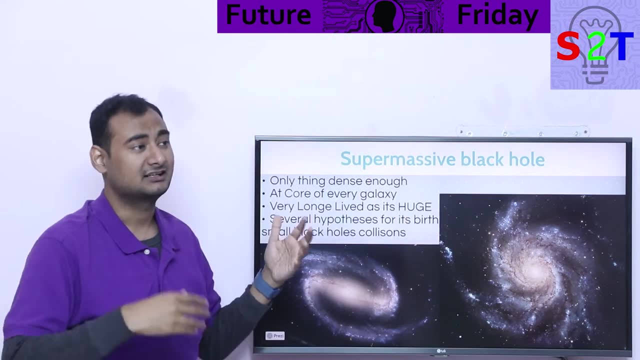 so it will start to remain in calm state for much longer and more it can absorb, so it becomes a self-fulfilling loop where it can grow, grow, grow and keep growing to super massive black hole size. there are other hypotheses that like in early- uh, like you know, early universe, where, after big band, 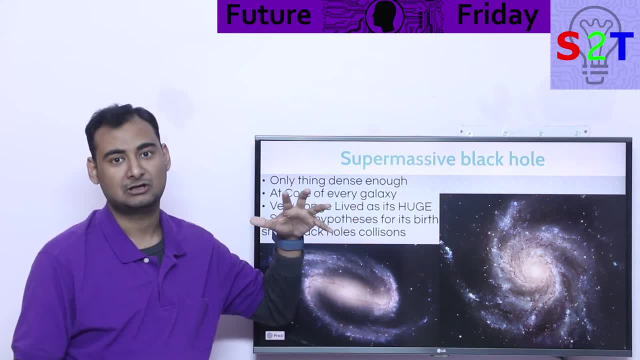 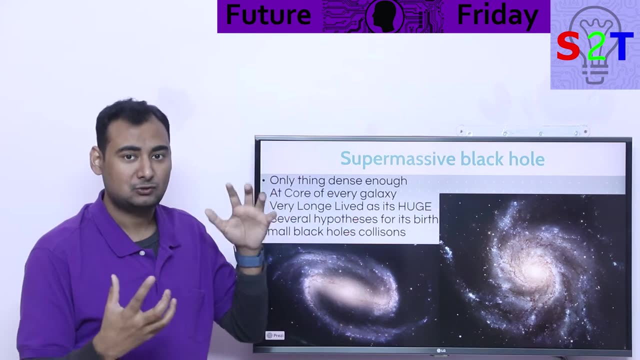 uh, as giant clouds, basically giant nebula, quote-unquote collapsed, and generally this is a normal thing. things collapse and make into a star. however, if it was too big from beginning, it will collapse so fast that it will not go into stellar phase. it will directly end up in black. 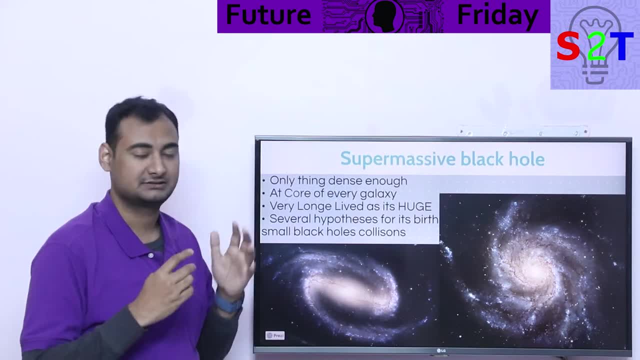 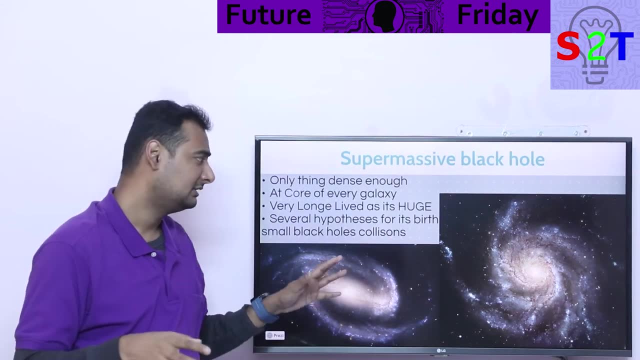 hole phase. that could be one way of reaching a point where you can just have a super giant black hole which might have a super. no, why not? but be mindful, these are hypotheses. there are many more hypotheses about this, like uh, last time i checked there are like seven to ten hypotheses about this. so but we know. 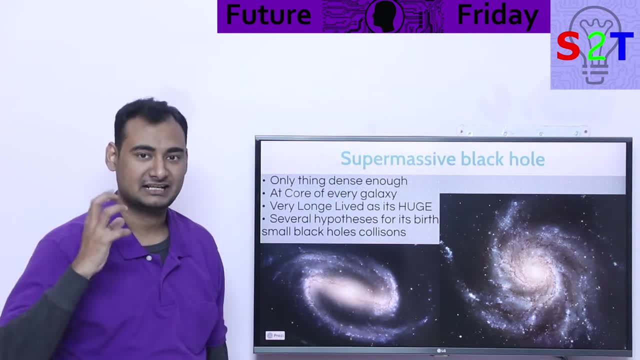 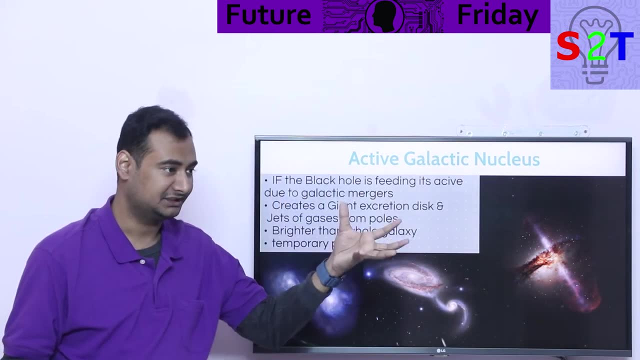 that there is a super massive black hole. that part is known. that's the only thing that can have that kind of influence. now we are talking about something bright, something that is brighter than the whole freaking galaxy. it's a milky way galaxy and this one thing has more energy than 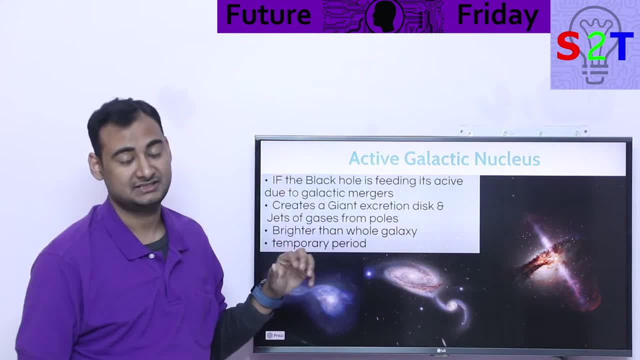 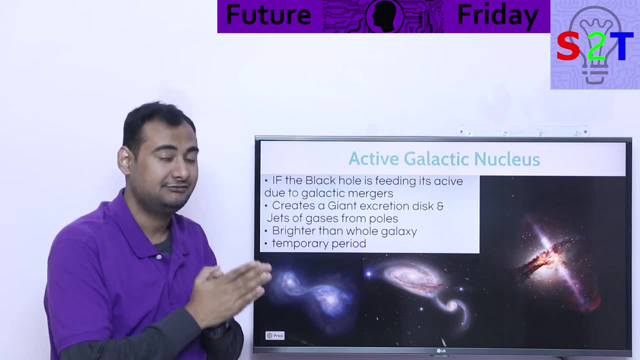 how the heck that can happen. that happens during the feeding era. basically, if the star is quote unquote active, which we call active collective nuclei, then this puppy is. that's why i specified the life of this is very critical because from its point of view it's like: oh dude, i ate it and, like you know, in the morning that would be like 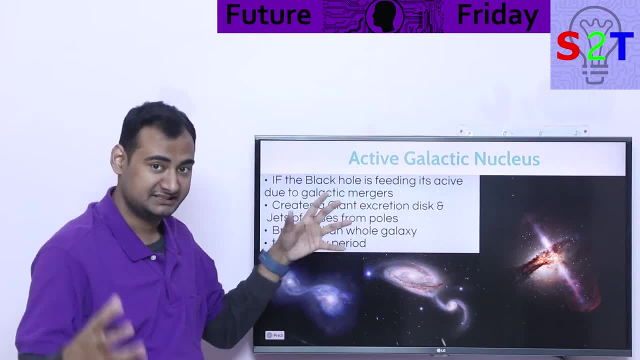 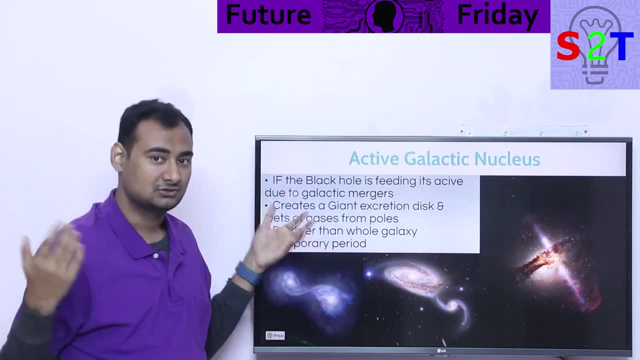 you know, 5 billion years ago. so when it's active, when it's actually feeding- basically it's being fed by multiple gas clouds, multiple, uh, basically stars, or like whole other neutron stars, black holes or whatever have you- it's feeding it. that time it creates accretion dicks. now how the heck you're? 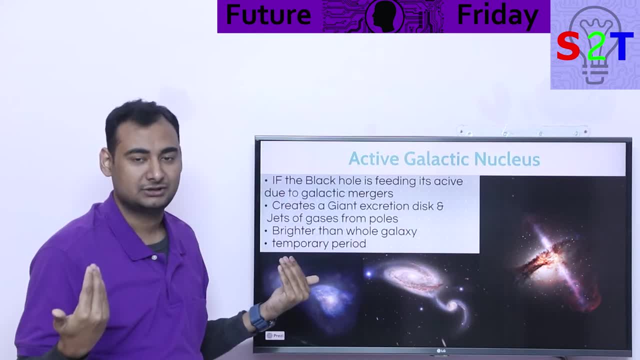 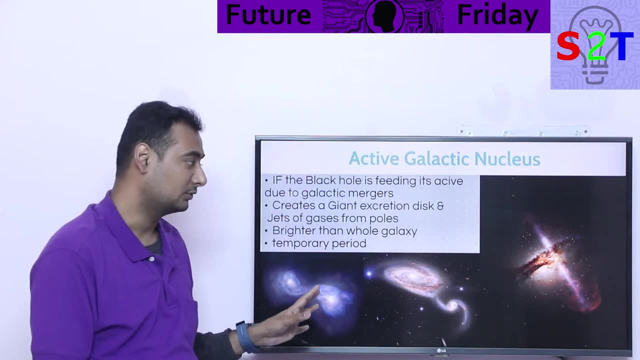 you're going to feed something this massive which has not already cleared this old quote-unquote galactic neighborhood. you generally collide with another galaxy like. these are normal things. this happens in the universe, quote-unquote, and we are also going to face this same fate simply because 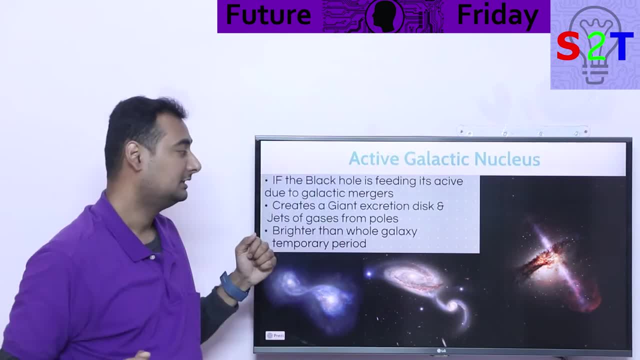 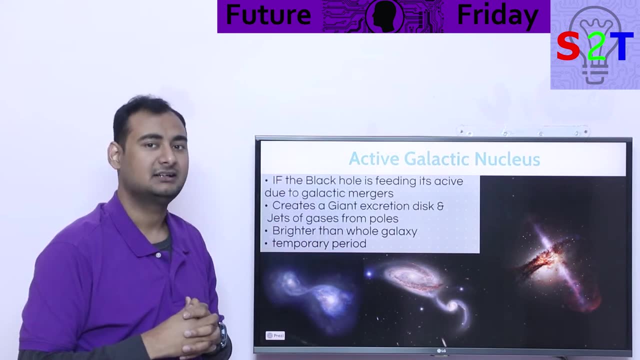 andromeda and milky way. they are in a collision course, so we're going to go like this now: most stars, they will pass each other without any issue. they will have gravitational influence, but they will not do much. however, galactic centers: yeah, they're gonna collide. it's not optional, it's. 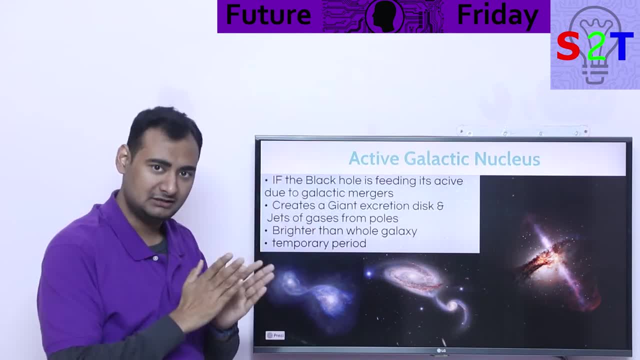 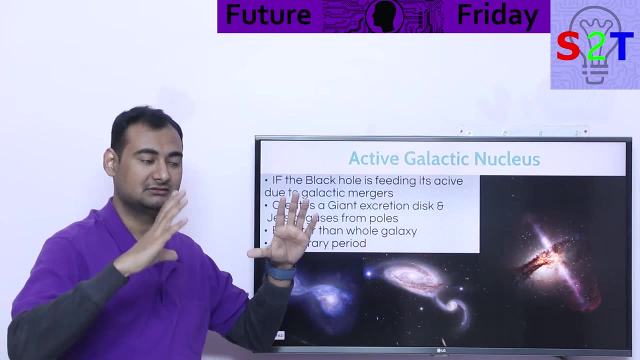 definite now how the heck they will merge. that depends like, of course they will merge. it's just how they're gonna merge and during that period, enough things will collapse that it will start to create this another active galactic nuclei. so the galactic nucleus that will become uh will have 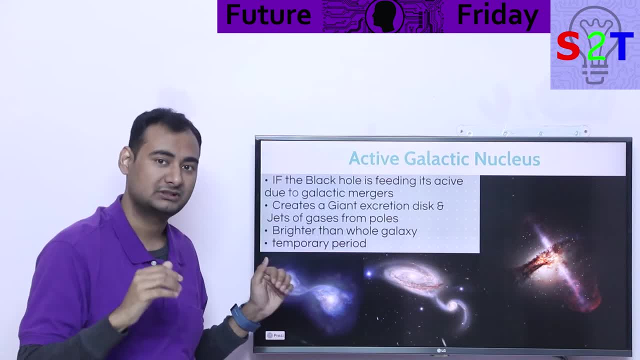 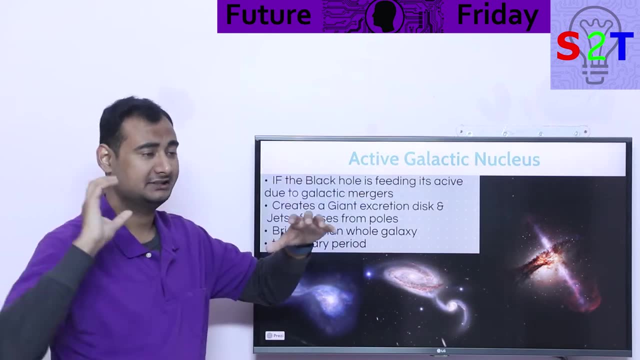 a active core, it won't have a calm core, the same calm core that we have at this point in time. now, because of the amount of energy it consumes, like, basically the expression is- it's ludicrously, it's like- the amount of speed those particles during, for, uh, like you know, particles, those 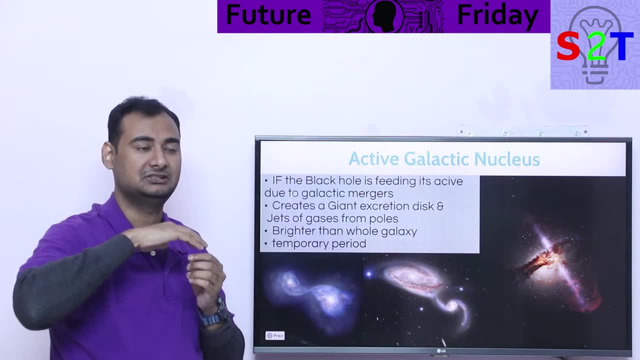 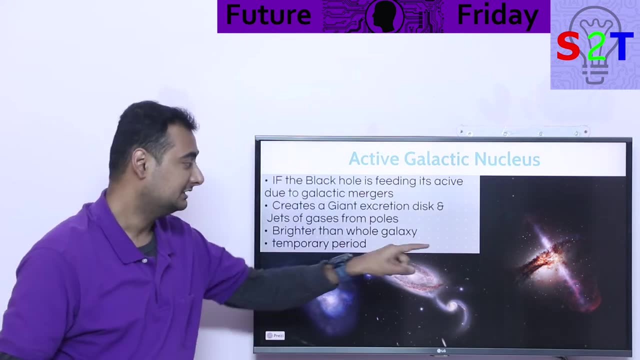 gain during falling into that. you know it's high, as in like it's so goddamn high that somehow starts to create weird, weird things, which includes x-ray emission, and if they are falling correctly, they may end up in a pole region, which does not even make sense. like how the heck that even happens and it it poles can be so powerful. 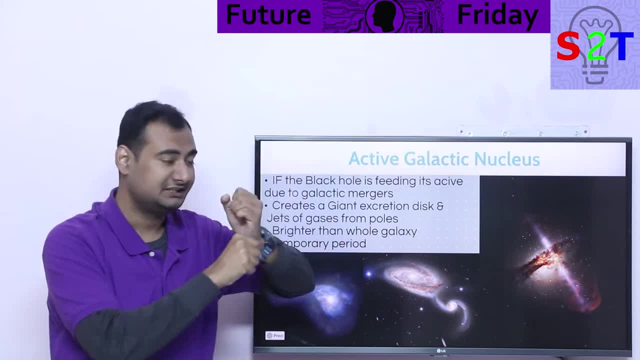 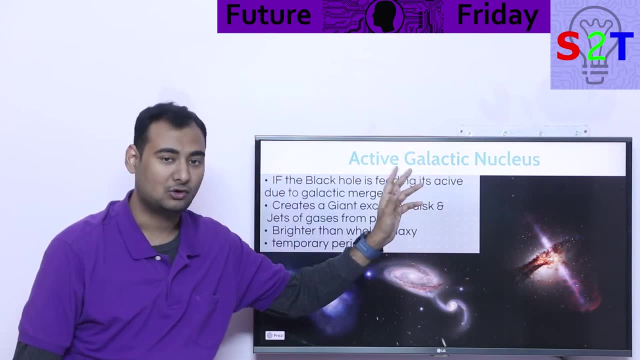 like the twisting of those magnetic fields could be so strong that it escapes. like think of this way. there is this star that has so much energy and yet somehow you can escape this, and the escape energy is so damn high. it's almost at light speed. basically, these jets they are traveling at. 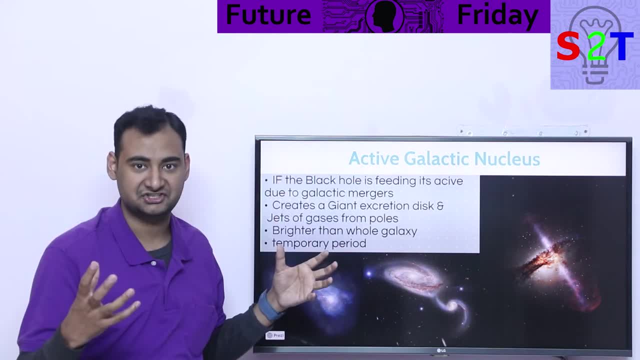 almost light speed, like we have something similar on our sun when we have solar mass ejections. but like those- uh, those are ludicrously fast. like we see them, light speed buys. it takes us eight and a half minute to know that they are coming and it takes like around 12 hours to few days to for them. 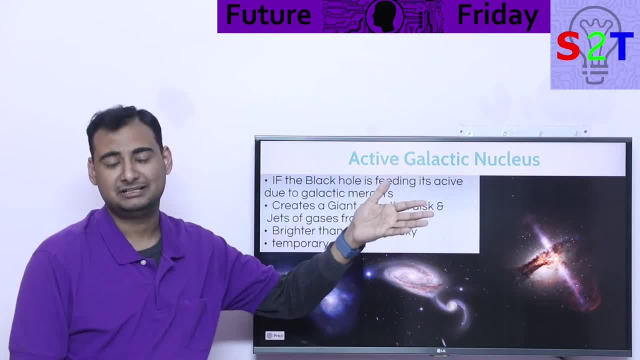 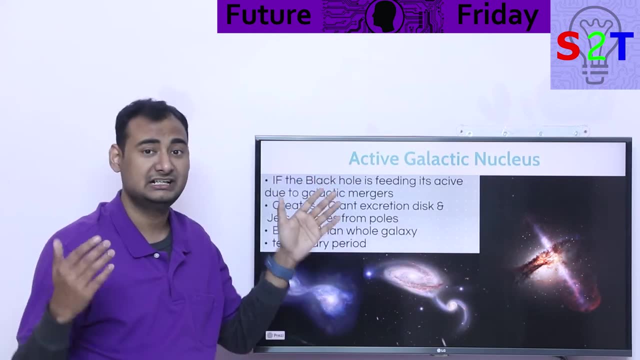 it to reach here this puppy. it will be like almost like if it's eight, uh, eight minutes a few seconds. it will be like eight minute half millisecond later. it's like that's how fast these things are. these are so fast they have realistic effects on applied to them, so it's ludicrously high energy. 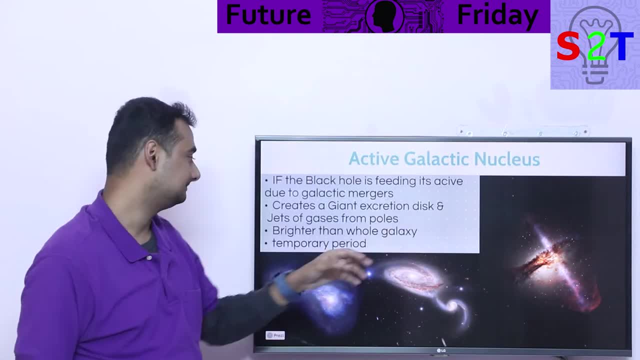 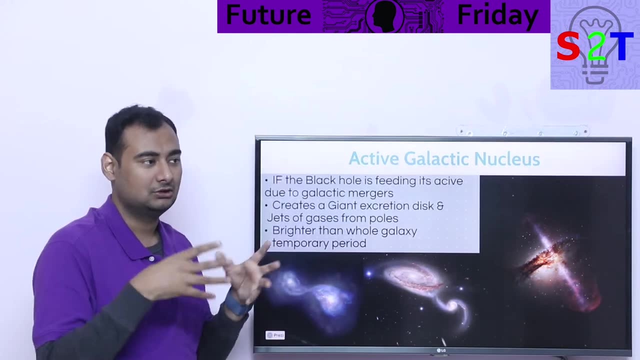 event that we are talking about. that's why it's classed as active galactic nuclei. now, at this moment when it's feeding, that point it's brighter than everything. that's why the age is so critical. it's not like, oh, it goes through phases, you know, at that point, when it's actually feeding, it's brighter than whole galaxy, and it is. 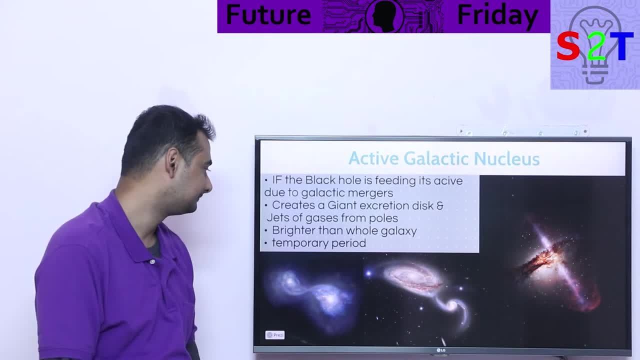 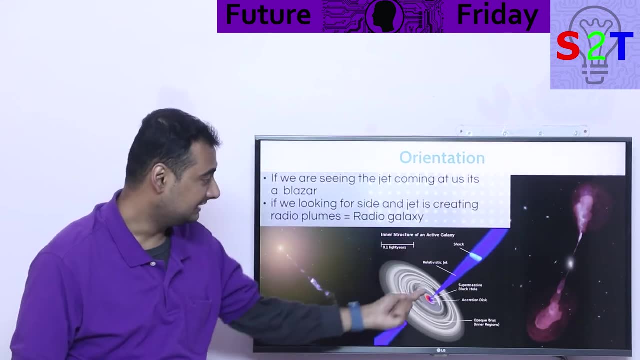 a temporary period, it's not something like it's gonna remain there forever. now, orientation of this thing: because of the high energy required and the fact that there is a disc and there are jets, basically poles of it, it has a very serious orientation bias towards us. basically, if we 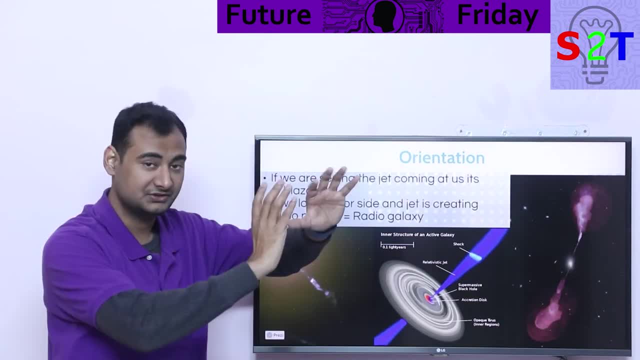 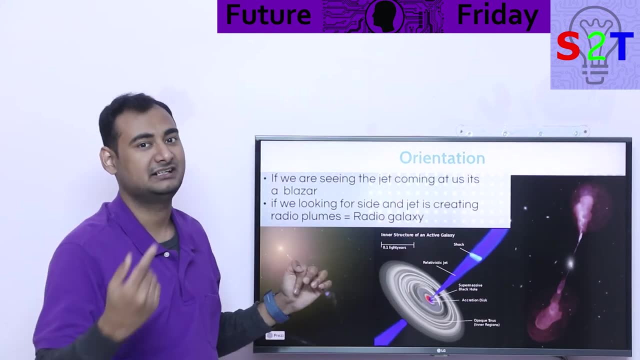 can see the pole side. basically, if the pole is facing towards us and we can observe it directly, we'll call it blazers. now, these blazers are ludicrously bright because, due to realistic effect, it looks much brighter than it actually is. now, be mindful, we are very lucky, all the brazors. 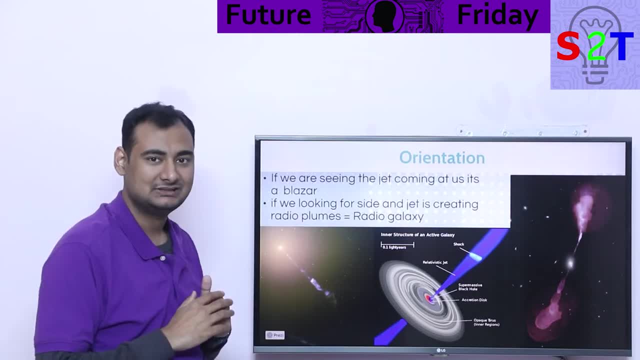 that we are observing. they are not very close to us, because if it was very close it will just whole solar system. so be mindful, that's the whole point. the orientation matters. so, uh, not all quasars could be blazers, but all brazos are quasars, so to say. and what will happen if you are looking? 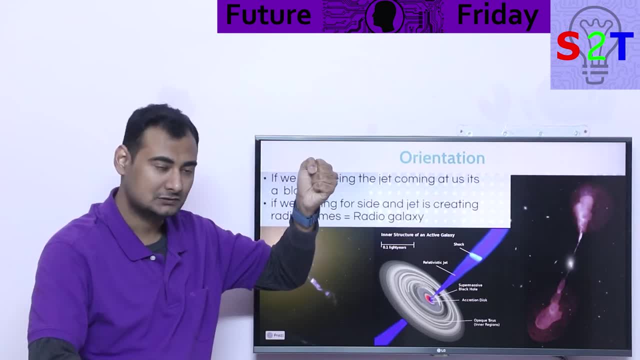 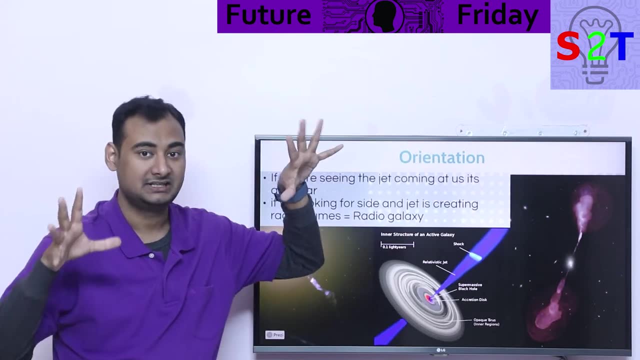 you're looking edge on. at that point in time, if it still has poles, uh, basically, pole is still excreting gases, because these are temporary also. uh, they will glow this whole area. this whole area will glow in radio waves and due to the glow and the brightness, we'll call it radio galaxy, and there, 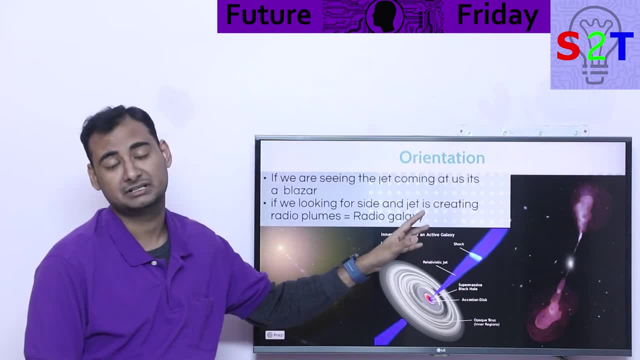 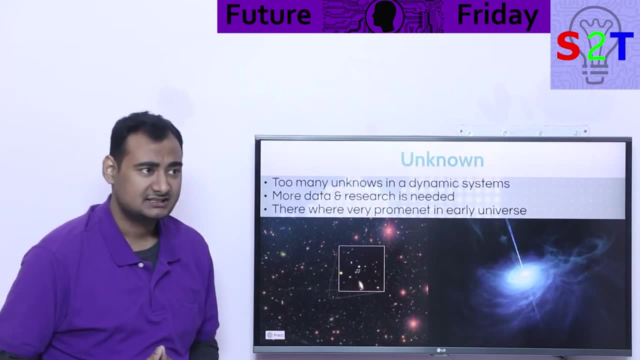 are many other subcategories also, so be very mindful. this is very orientation dependent how you are seeing it. that's how we classify it. now you have to understand quasars is one of those things that, like, we are just unlocking. it's like, oh, now we can see it. oh, now we can see this. this. 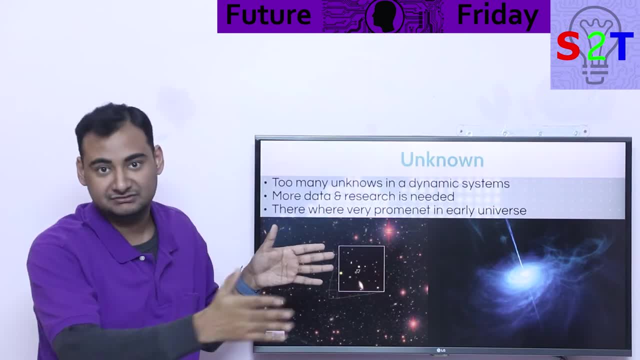 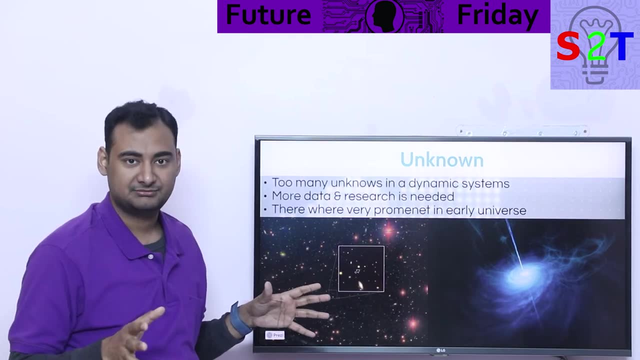 10, 20 of these. oh, now we are seeing like it has this kind of mass range when supermassive black holes are considered. uh, this kind of energy output we are talking about. so this is ludicrously un. uh, you know, variable system, where it has multiple variables and all of them are dynamic systems. 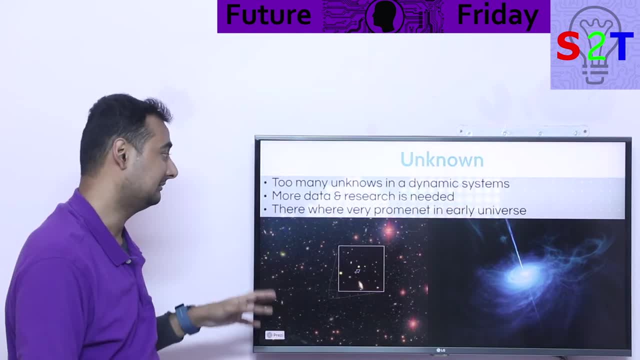 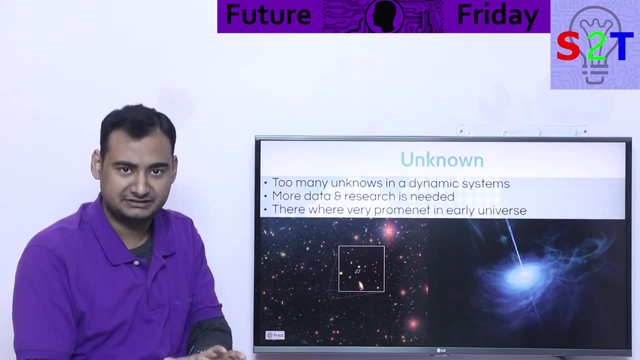 so, fundamentally, we don't have enough information at this point in time, so we need a lot more data and a lot more research before we can be like okay, like how we know about planets is like we know, this is a planet, we got this. like we, we got this. stars, we got this, even black holes we understand. 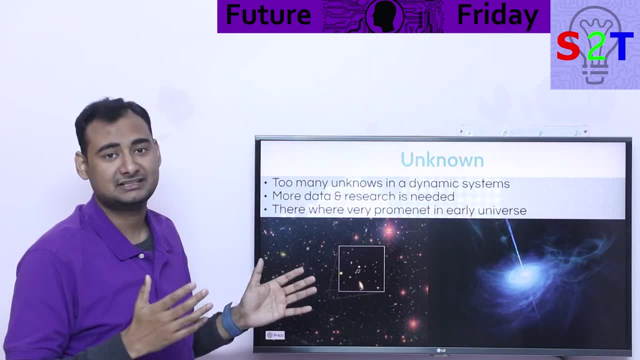 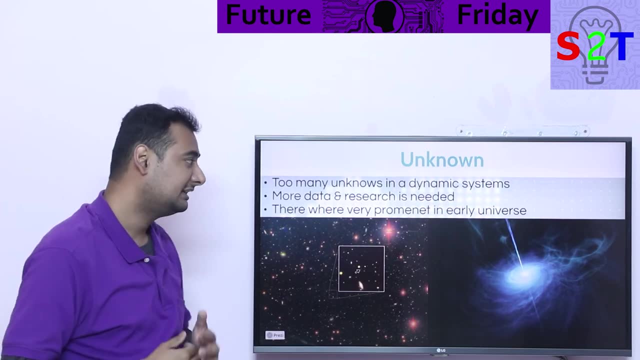 very large extent, but this probably is on a whole different level and it is complicated by the fact that it's a temporary phase of a super massive black hole. so all those things consider it's a very complicated puzzle and there are very, uh strong indication at this point in time that these things were very common average in earlier universes, basically when universe was very young, that super massive glass giant that is collapsing directly into black hole was much more easier to achieve and not to mention early universe already had like super massive uh stars and those stars have much higher probability of becoming into black hole. those black holes have much higher